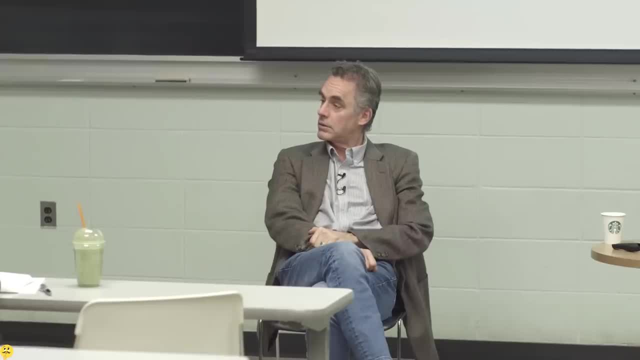 Oh, But I still found it. It's still in 430.. Oh, okay. Well, there's an essay. oh, that's too bad. It's not on the Psych 434 website, even Because I updated it. Anyways, I have this guide to writing. that's that if it isn't on the 434 website, it is definitely on the 430 website. 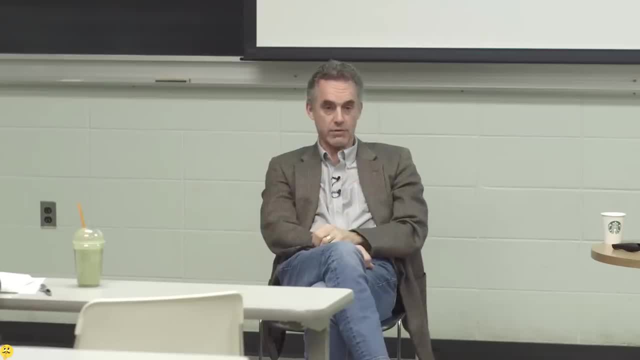 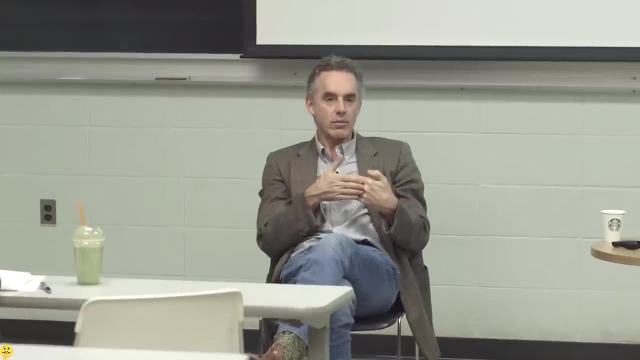 And it steps people through the process of writing. Because what's happened now? it's very hard to teach people to write because it's unbelievably time intensive And like writing marking a good essay, that's really easy. Check A. 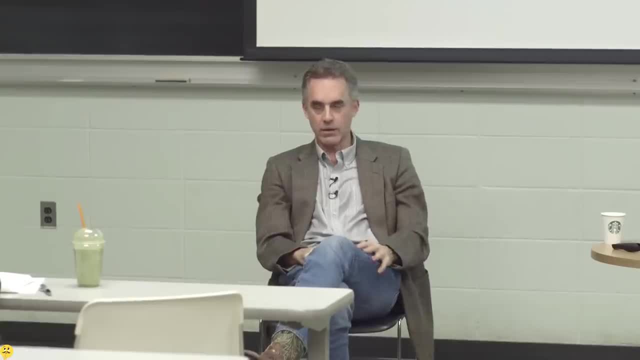 You did everything. You did everything right, Right Marking a bad essay. Oh my God. The words are wrong, the phrases are wrong, the sentences are wrong, they're not ordered right in the paragraphs, the paragraphs aren't coherent and the whole thing makes no sense. 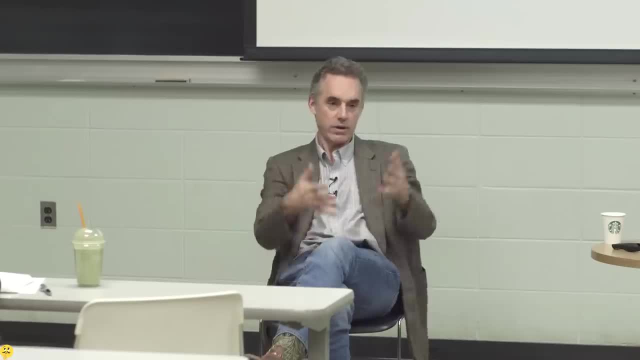 So trying to tell the person what they did wrong, it's like: well, you did everything wrong, Everything about this essay is wrong. Well, that's not helpful either. You have to find the few little things they did half right and you have to teach them what they did wrong. 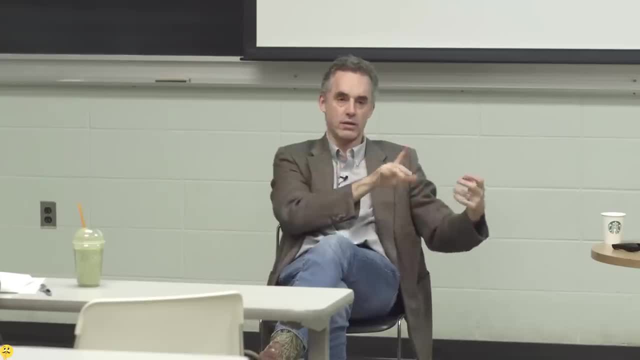 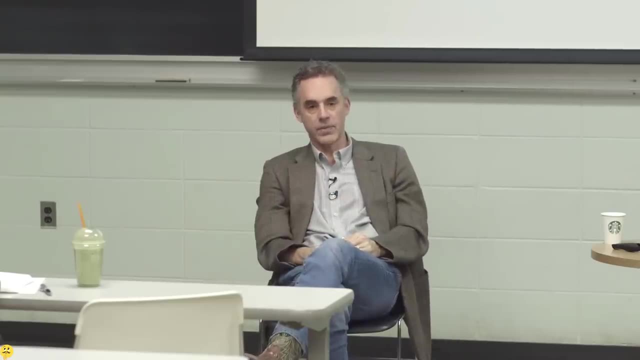 It's really expensive. What I did with this rubric was try to address that from the production side instead of the grading side. But the best thing you can do is teach people to write, because there's no difference between that and thinking, And one of the things that just blows me away about universities is that no one ever tells students why they should write something. 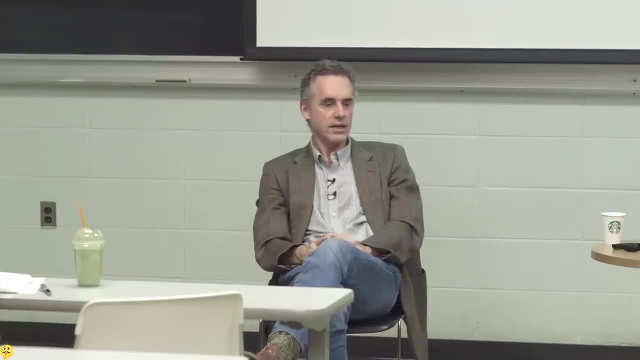 It's like: well, you have to do this assignment. Well, why are you writing? Well, you need the grade. It's like: no, You need to learn to think, Because thinking makes you act effectively in the world. Thinking makes you win the battles you undertake. 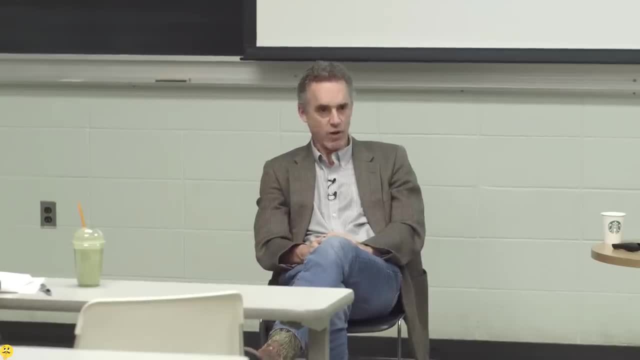 And those could be battles for good things. If you can think and speak and write, you are absolutely deadly. Nothing can get in your way, So that's why you learn to write. It's like I can't believe that people aren't just told that. 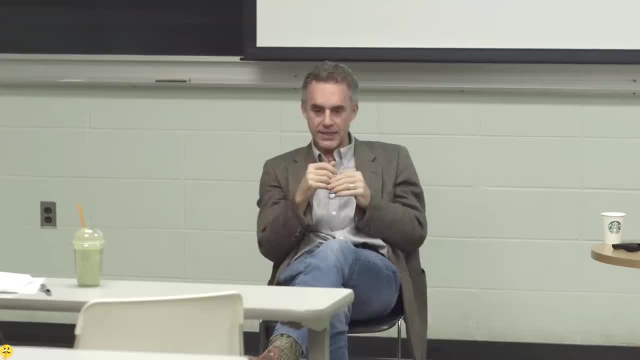 It's like it's the most powerful weapon you can possibly provide someone with. And I mean I know lots of people who have been staggeringly successful and watched them throughout my life. I mean those people you don't want to have an argument with them.